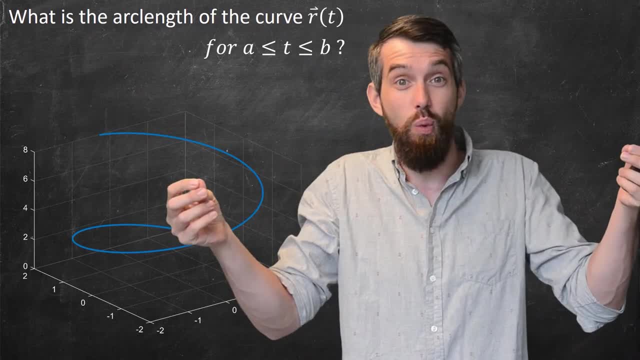 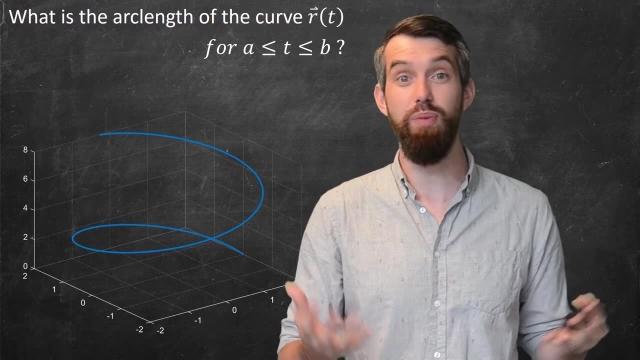 curve which is made out of string, and I took the string and I stretched it out. well, how long would that be? In general, if I have such a curve, I usually don't know what its length is going to be, unless it's something really nice like a straight line or a circle, where I can say what the 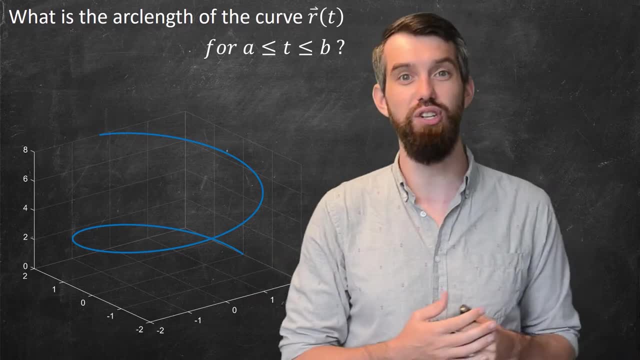 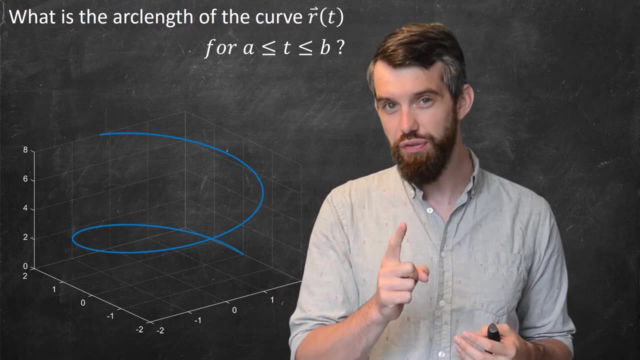 circumference is, But with calculus, as long as our curves are sufficiently nice and differentiable, then we're going to be able to compute their arc lengths. There's a couple steps to this process, and the first of them is to approximate this with straight lines. So what I'm going to do is: 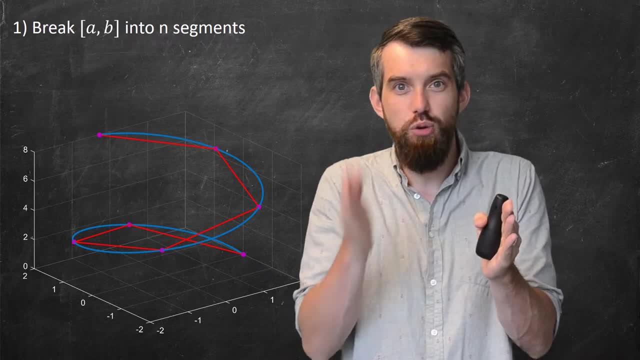 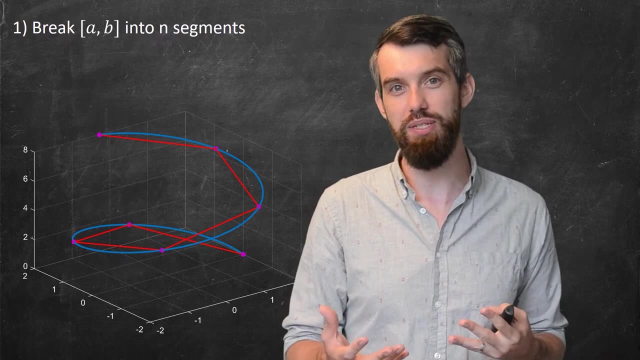 I'm going to take that a to b interval and I'm going to break it up into n equal-sized segments. So my parameter has been divided up into these n different segments, And then on the graph I'm going to plot where those points are going to go and I'm going to draw a line. 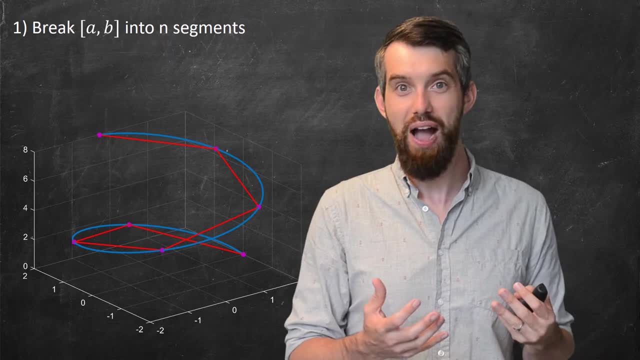 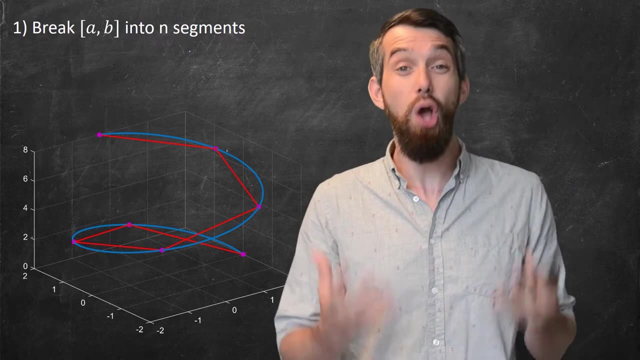 segment between all those points. So in this case I've divided the curve into six different line segments. The reason why I'm doing this is that I know how to compute the length of straight lines, So if I can approximate this curve with straight lines, 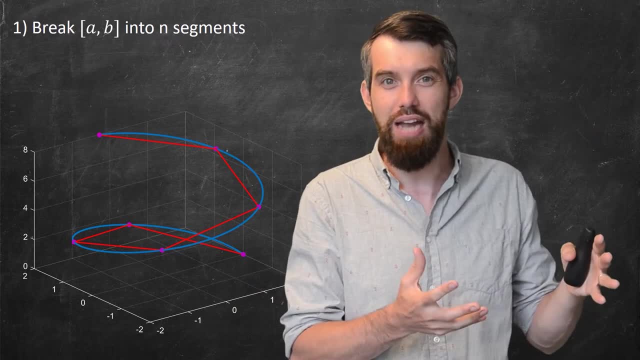 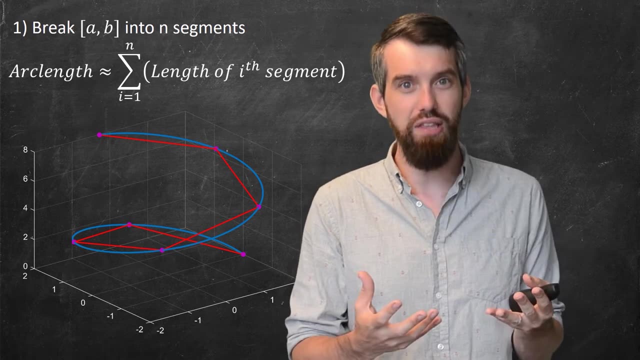 and I can go off and compute all the lengths of those straight lines. then I get an approximation for the entire curve. That's going to be our plan. So the first thing to note here is that the arc length of the original curve is not exactly equal. 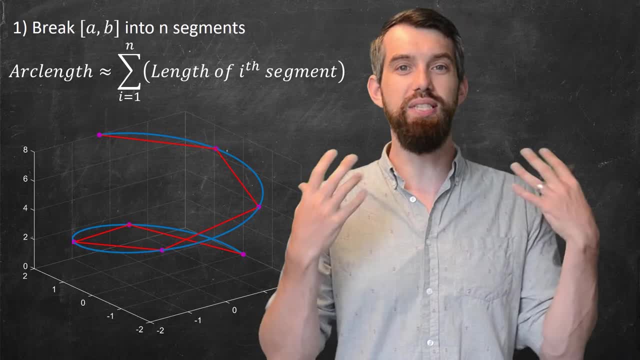 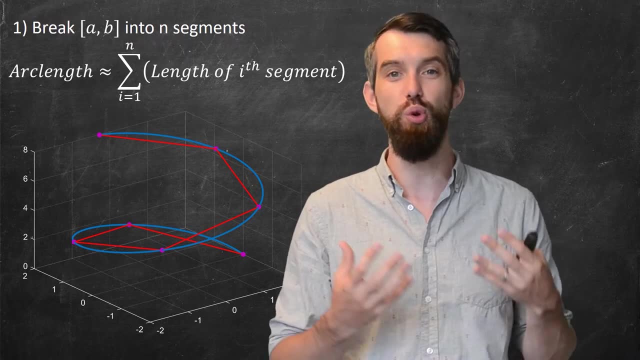 but it's approximately equal to the sum of all of these segments, the line segments. In this case I've drawn the six of them, But in general you'll write it from i, equal to 1 up to n. You take the sum of all of those arc lengths. 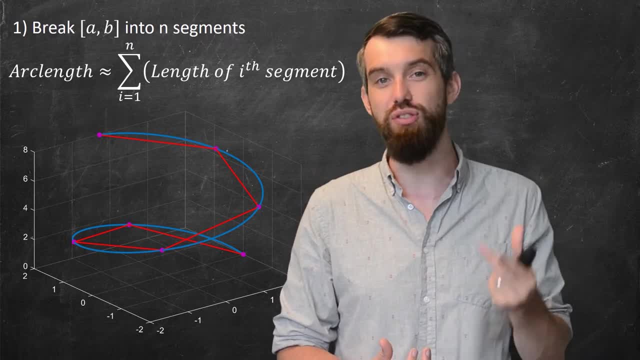 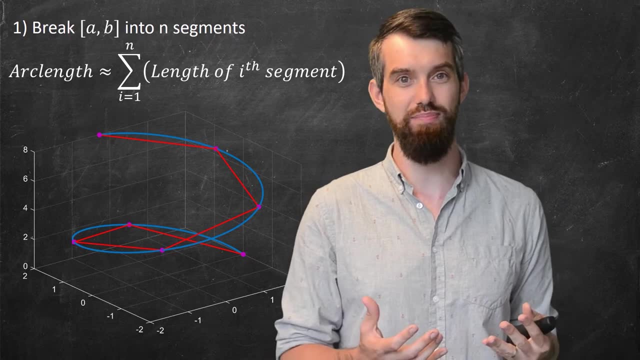 the first straight line, the second straight line and, generically, the i-th straight line. Now the problem, you might say, is: well, hold on, how good of an approximation is this really? It looks okay, but certainly there's a lot of difference between these straight lines and these curvy segments. 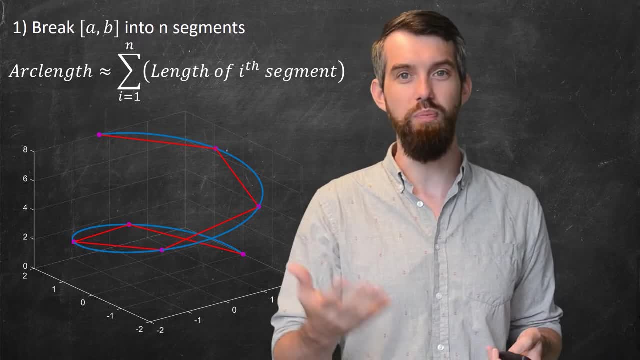 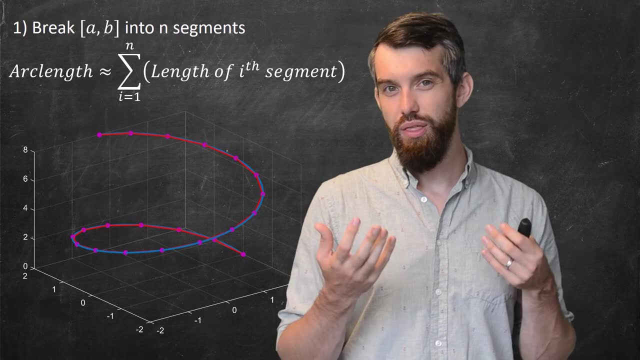 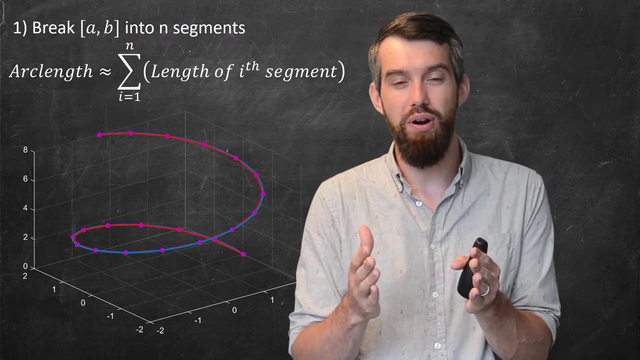 But what if I divide it up into more and more pieces? So instead of n equal to 6,, what if I did n equal to 8,, or n equal to 10, or n equal to 12, and so on? The larger my n is, the more ways that I break up that interval in the t parameter. 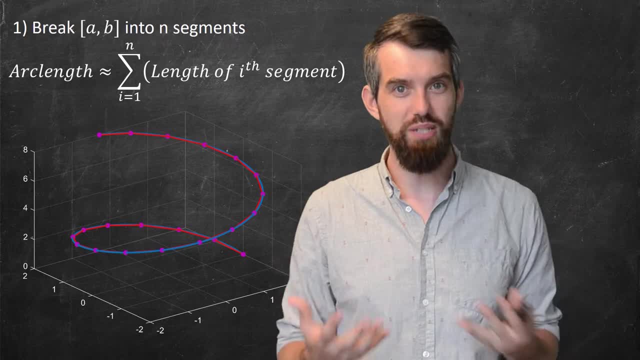 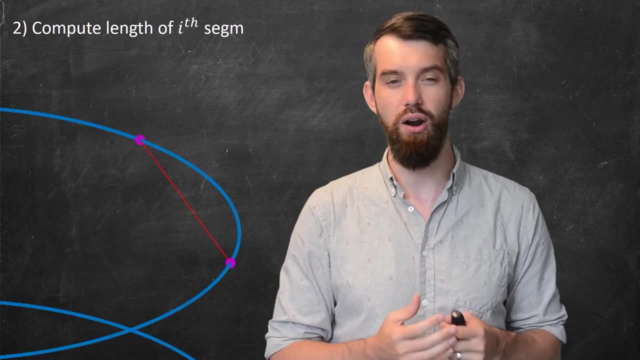 the closer and closer and closer. it appears that my approximation is getting to the original thing. Okay, so, with that big idea stated, let's actually zoom in a little bit here on one specific one of these straight line segments and try to figure out: well, how big is that? 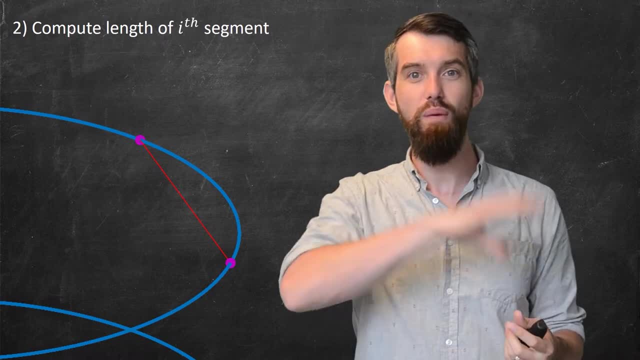 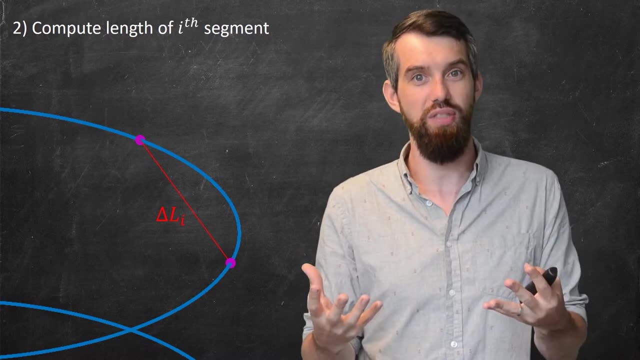 How can we compute that? In particular, of all the multiple different line segments, this is one of them and I will call it delta li. So it's the i-th change in the arc length going between a pair of points. Okay, 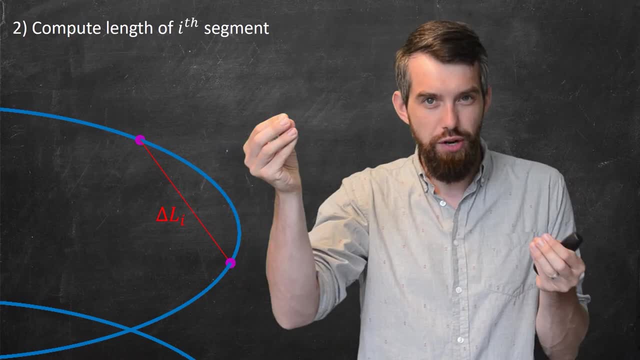 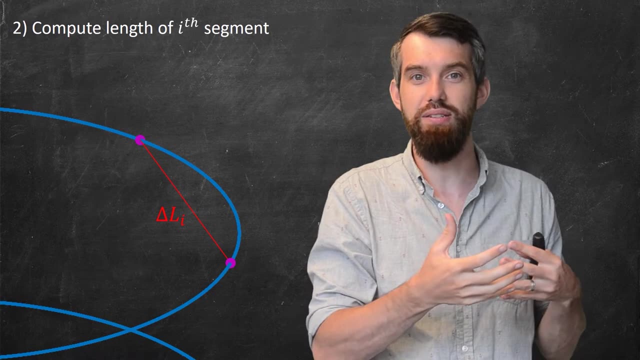 Now, if I think about this, I've got my curve, I've got these two different points, I've got the straight line between them and these two points have a difference in x, in y and in z. So I can put that on my plot. I can say there's a delta xi, a delta yi and a delta zi. 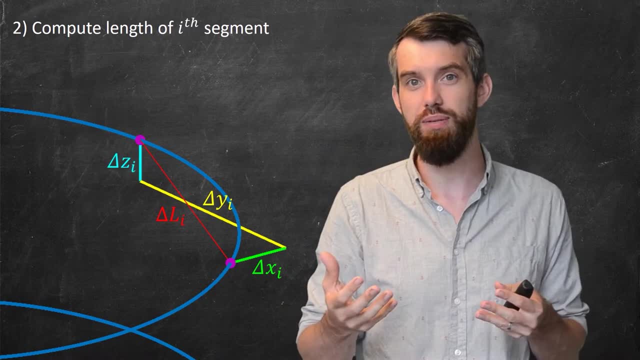 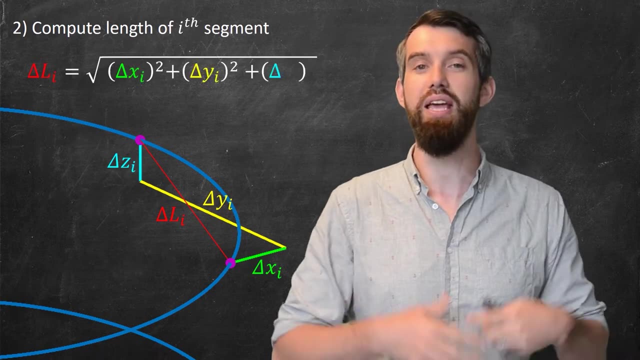 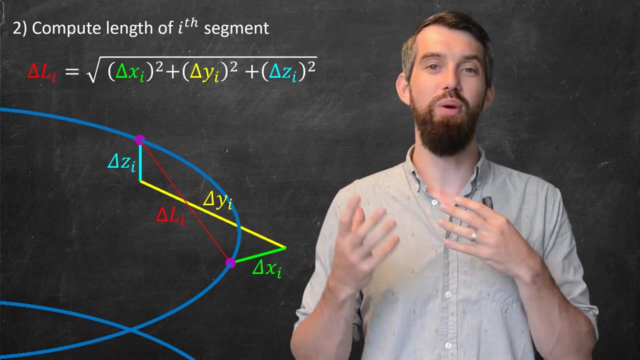 So my two points differ in all three components. But now I can say what the length of the straight line is. That's just a Pythagorean formula. Namely, the delta li is equal to the square root of the delta xi squared plus the delta yi squared plus the delta zi squared. 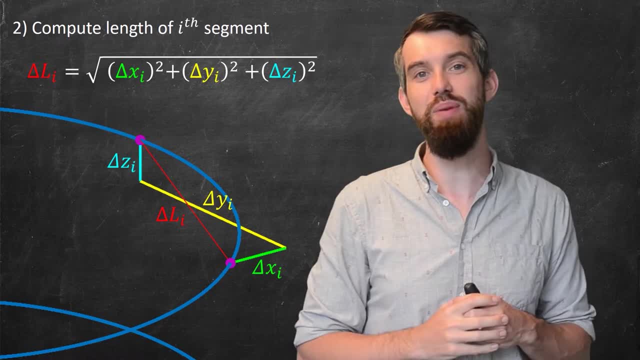 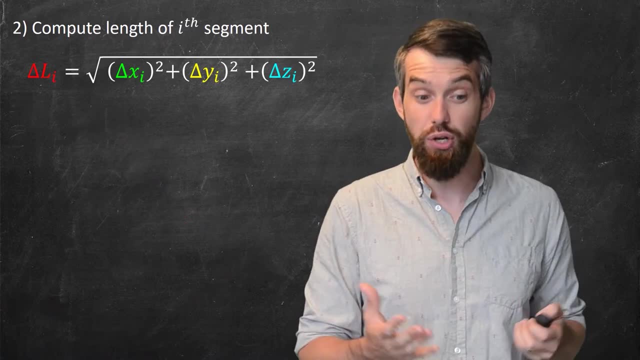 So we've zoomed in on the generic i-th segment here, We've figured out what its length is in terms of sort of x, y and z, And now let's put them all together. So, going back to our original computation, where we said arc length was the sum of these little line segments. 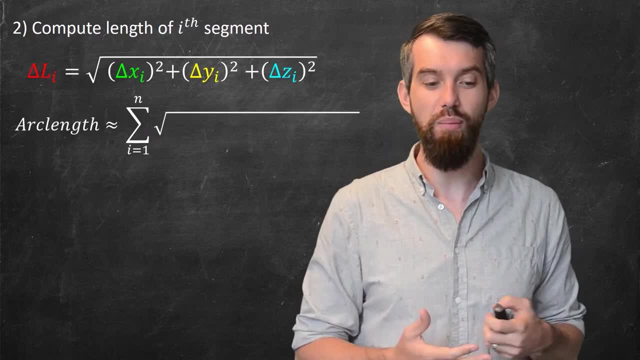 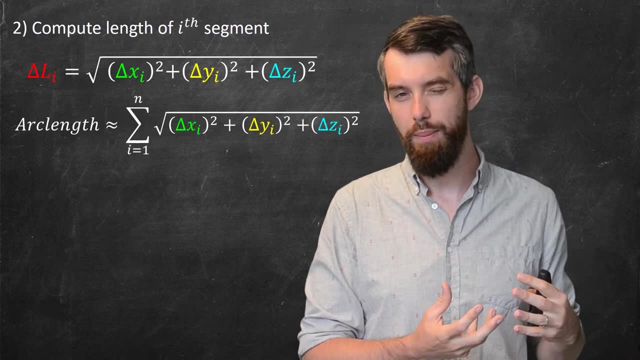 Well, now I know what the delta li is. so it is the sum of the square root of the delta xi squared plus the delta yi squared plus the delta zi squared. Okay, now pay attention, because I'm going to do a little bit of a trick. 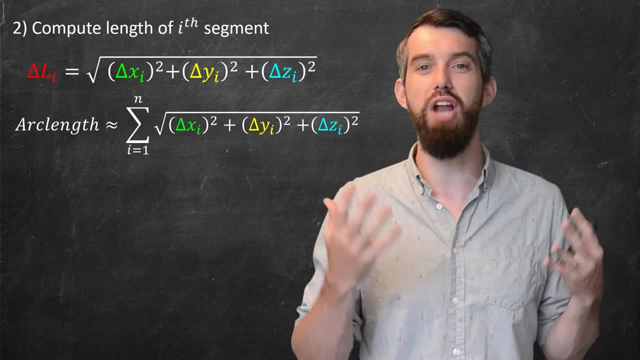 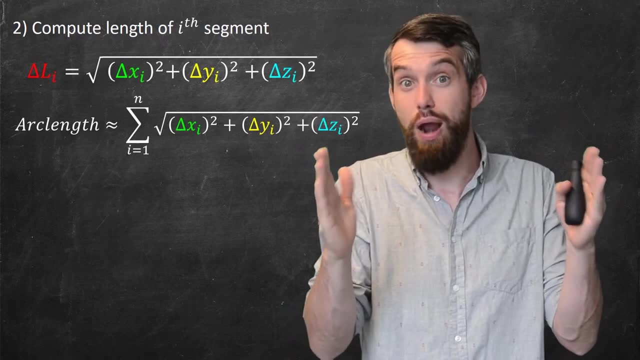 I'm going to multiply this by a funny version of 1.. Remember how we took the original interval a to b and we divided it up into n little segments in the parameter t. So the width of each of those little segments in the parameter t was, let's call it, delta t. 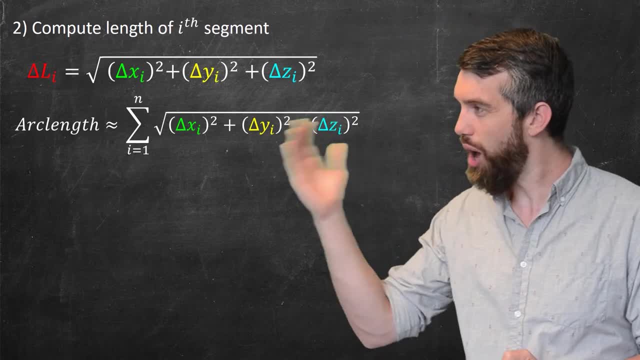 So what I'm going to do here is I'm going to multiply the top and the bottom by delta t- A funny version of 1, I'm allowed to do that. Then I'm going to take the delta t. that's on the bottom. 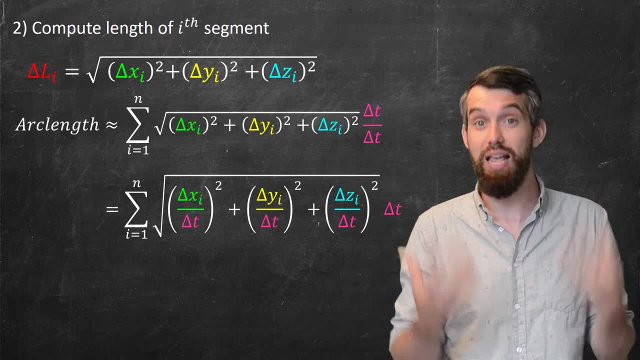 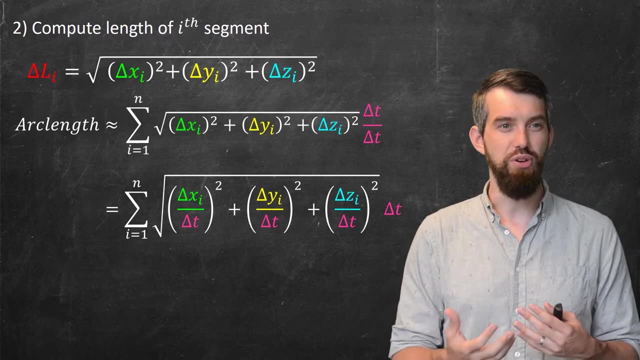 and I'm going to move it inside of the square root and inside of the square, so it's the delta xi over delta t, all squared and so on. Now the reason why I'm doing this- delta xi over delta t- sure looks like the derivative of the x component with respect to t. 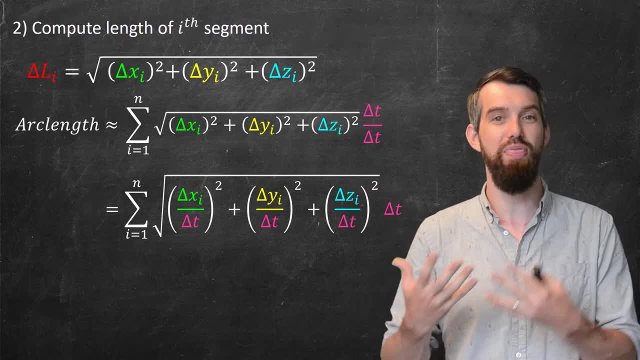 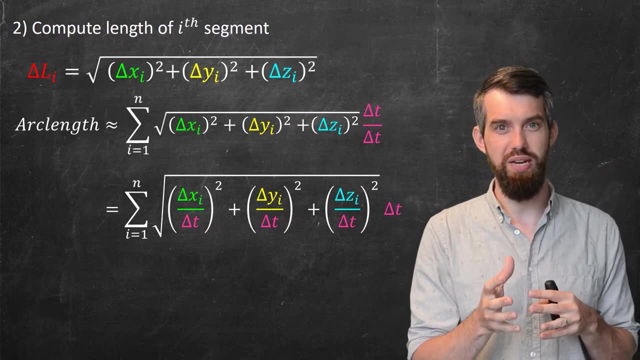 likewise for y, likewise for z. it's just that I'm not yet at the point of taking derivatives. I'm still doing finite deltas, Alright. so the next big move in my argument is notice how I'm saying. arc length is approximately this: 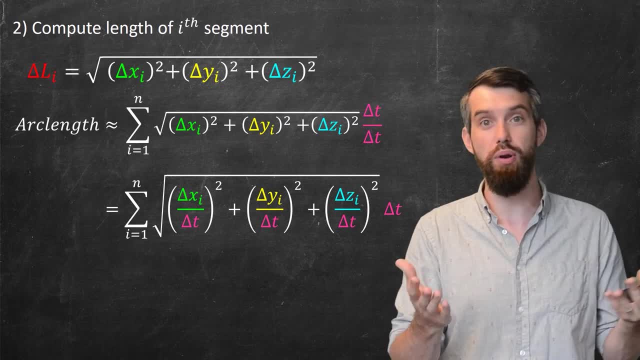 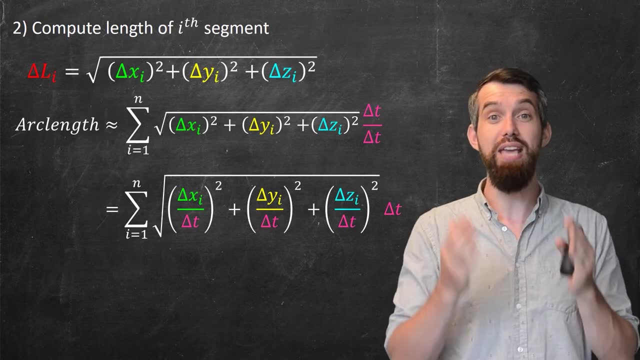 Because any n? I'm doing an approximation. I've only broken it up into n different components. But if I want to make it equal to it, if I want to come up with a definition, what I'm going to do is I'm going to take my delta t and make it smaller and smaller and smaller. 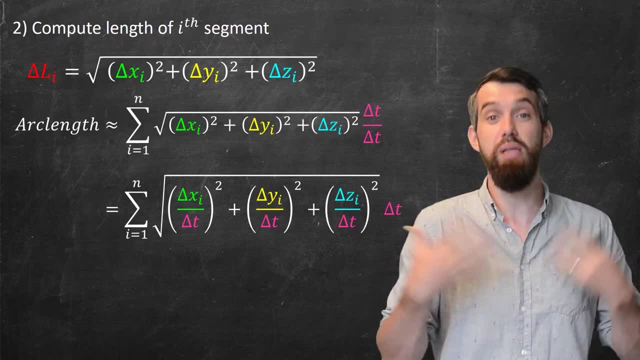 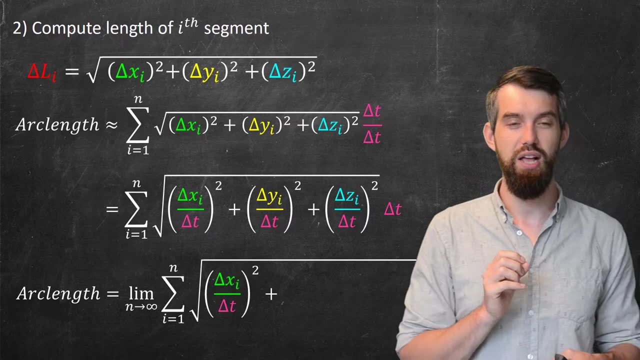 or say it differently, the number of segments is going to be larger and larger and larger. So let me replace the approximation with an equal sign and I'm going to stick a limit out the front of this. The arc length is equal to the limit, as n goes to infinity. of this summation that I had before, 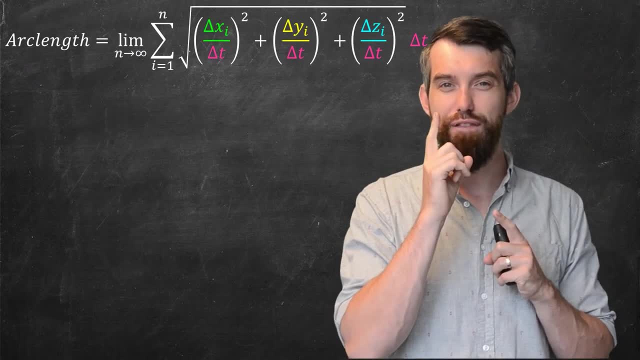 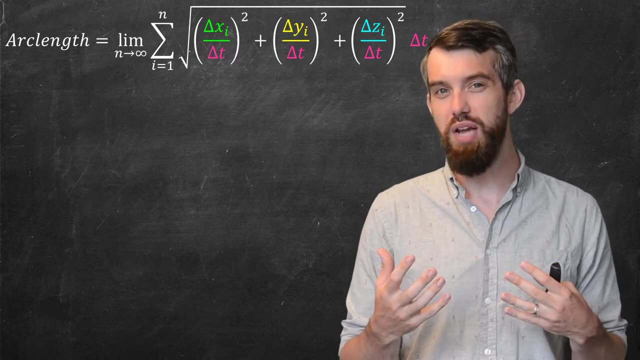 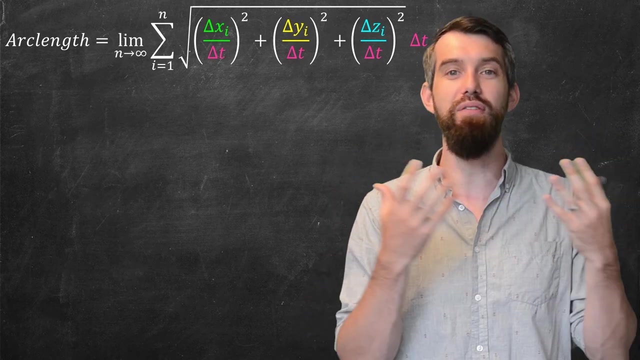 Moving this up, I'm now going to do my final thing, which is replace this collection of symbols with an integral, And you may recall that we've done this many times in the past, and indeed, when we thought about what integration was defined to be, it was the limit of a sum of a bunch of areas. 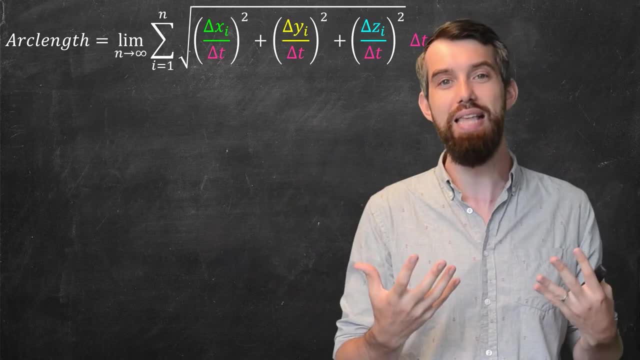 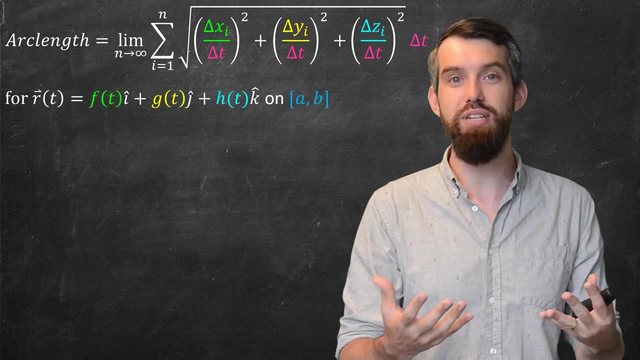 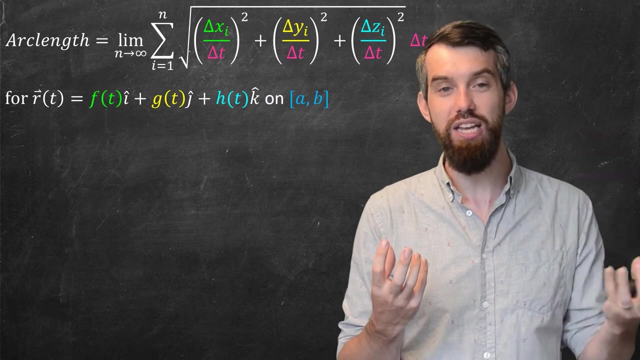 So, again here, I have a limit of a sum and I'm going to replace that with an integral sign. Before I jump into changing to the derivatives that are going to come out here, I'm going to set the notation That my vector value function r of t. I'm going to call f the x component, g the y component and h the z component. 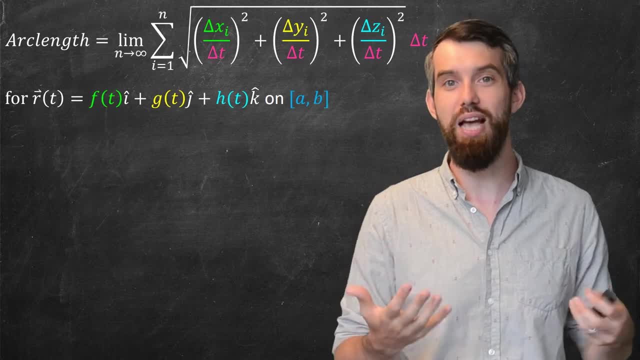 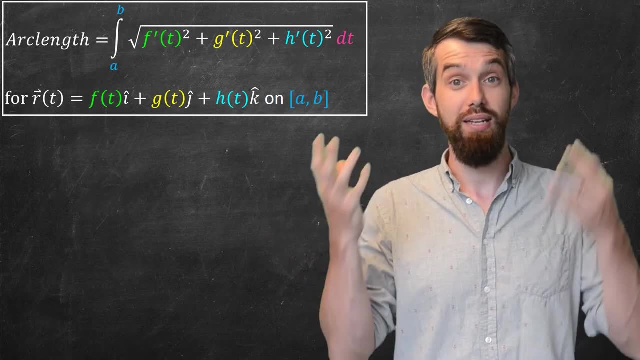 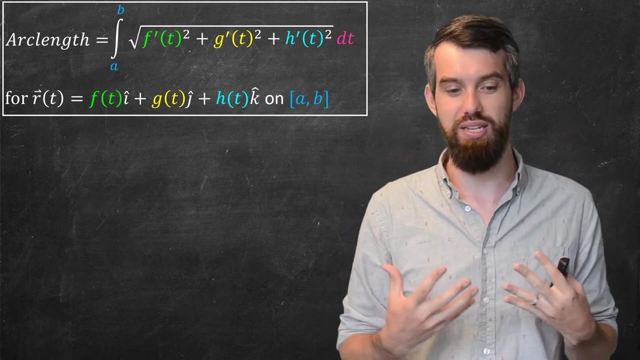 Well then, when I go and I take my limit of the sum, replace it by an integral, what do I get is the square root of the derivative of f. That's what happened when the delta xi over delta t. it got replaced in the limit with the derivative of f with respect to t or f prime. 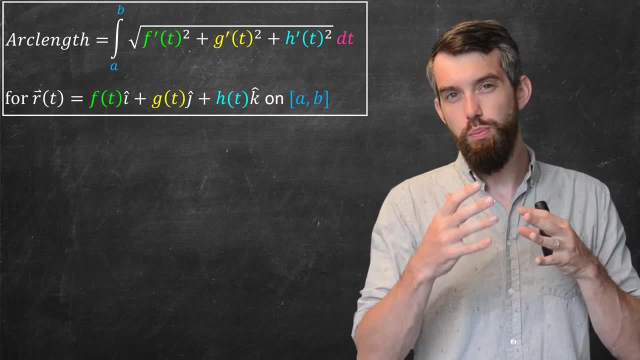 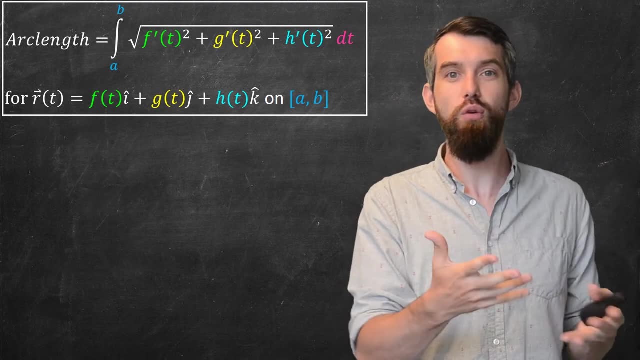 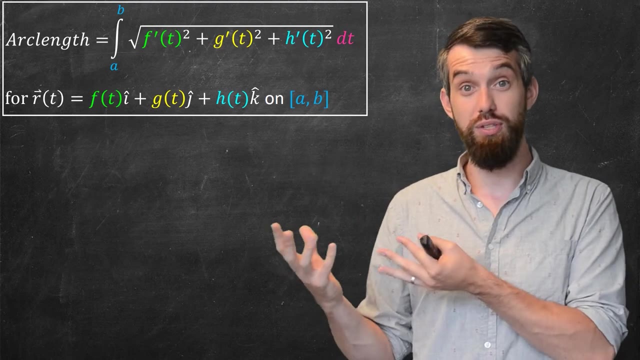 Likewise for y, likewise for z. So, provided my vector value function actually is differentiable, I can compute these derivatives. then, for any one that you might give me, I can just plug them into this formula. And sure, this formula is an integral, which means that for a lot of integrals,